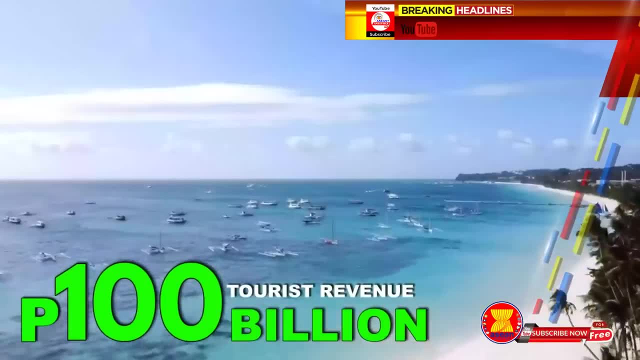 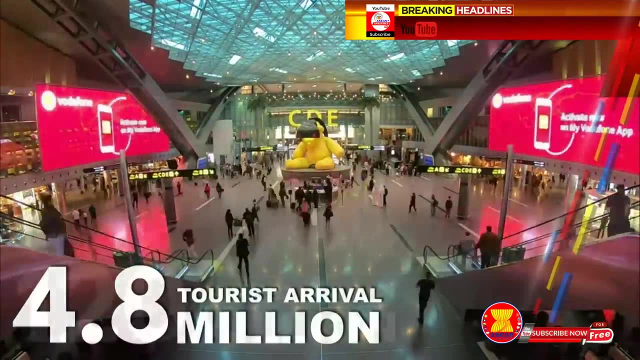 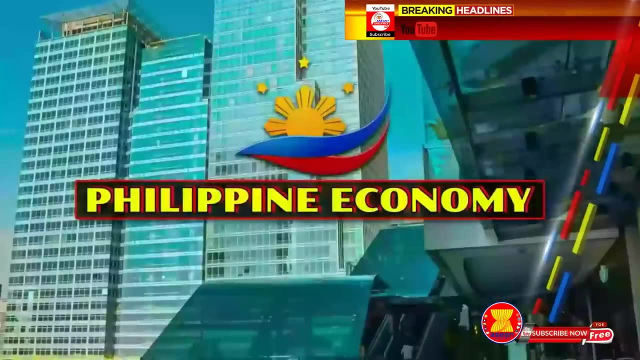 And these accounted for more than 100 billion pesos in estimated visitor receipts. For 2023, the Department of Tourism expects 4.8 million international arrivals and more than 120 million domestic trips. The Philippines has been one of the most dynamic economies in the East Asia-Pacific region. 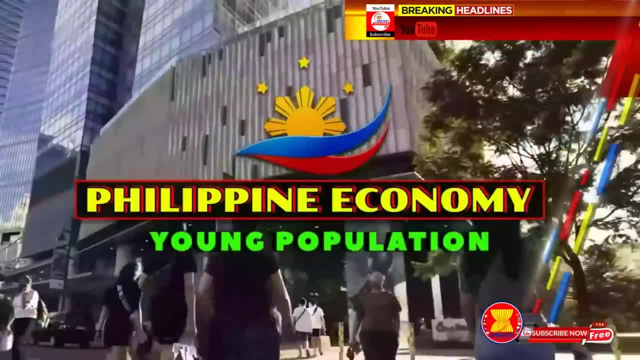 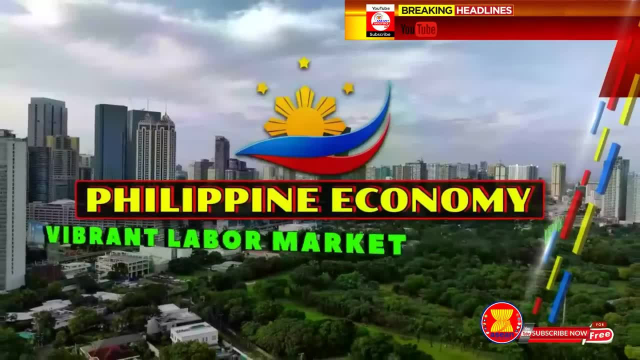 With increasing urbanization, a growing middle class and a large and young population. the Philippines' economic dynamism is rooted in strong consensus. The Philippines' economic dynamism is rooted in strong consensus. The Philippines' economic dynamism is rooted in strong consensus. 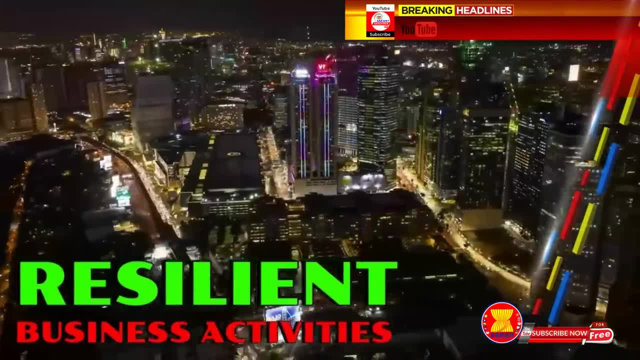 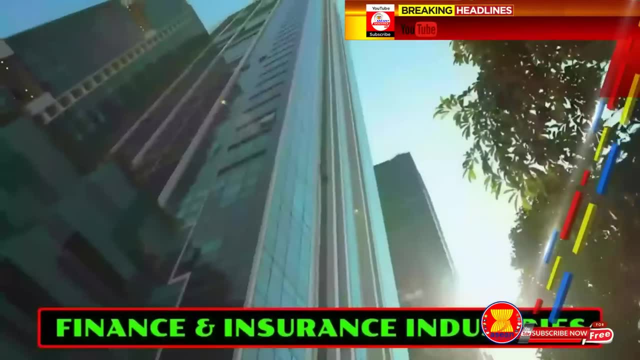 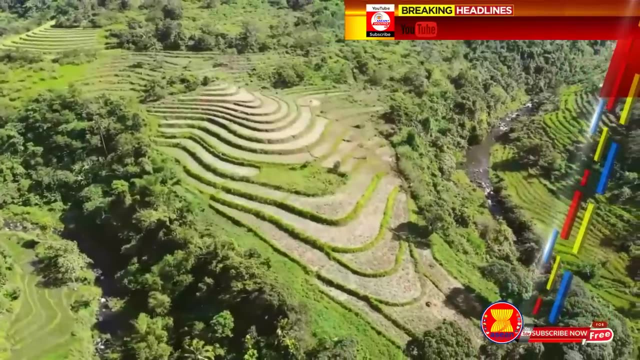 Business activities are buoyant, with notable performance in the services sector, including Real estate, Tourism, And finance and insurance industries. As a newly industrialized country, the Philippines economy is in transition from one based on agriculture to services and manufacturing. The Philippines' economy is in transition from one based on agriculture to services. 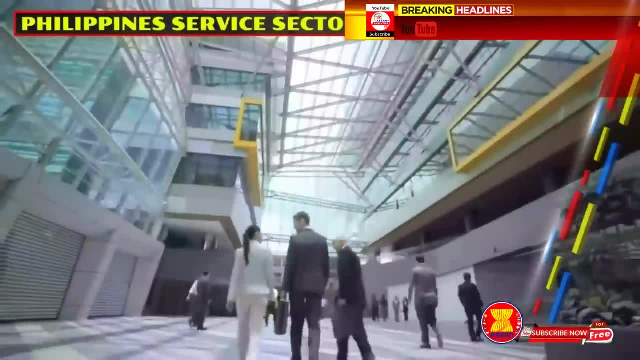 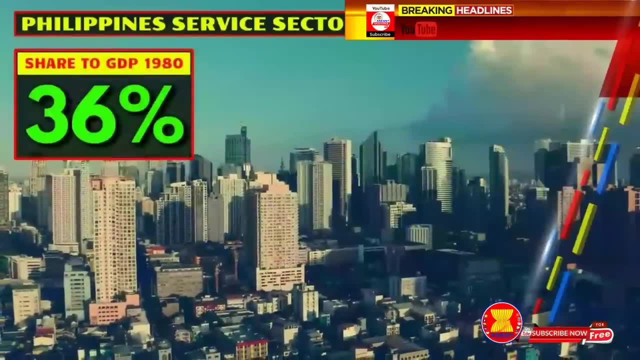 and manufacturing, And it is time to report on the outcome of demand growth in the partners of the United. The services sector of the Philippines overtook the industrial sector in terms of contribution to the GDP during the early 1980s, increasing from 36% in 1980 to more than 61% as of 2022,. 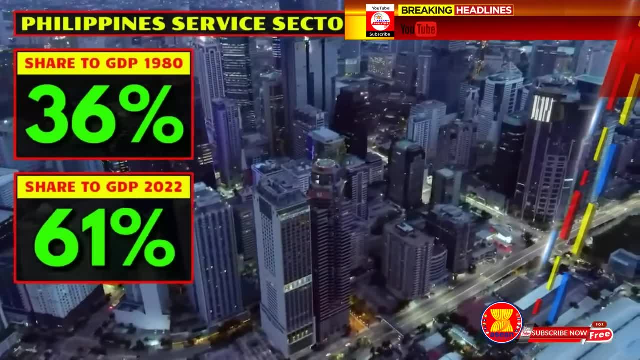 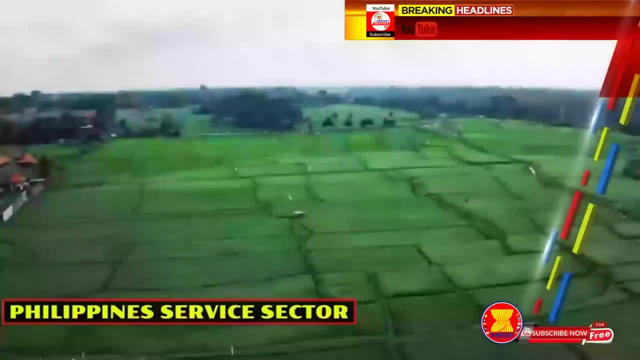 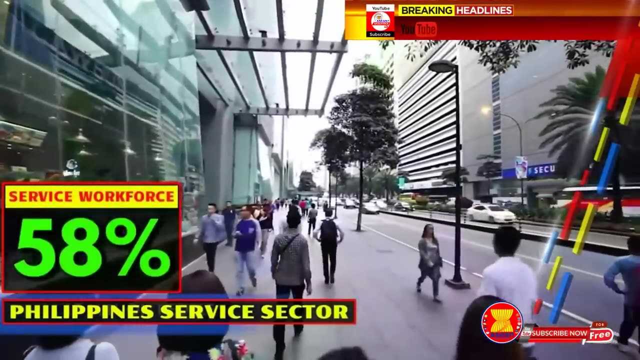 which was higher than the 60.5% share recorded in 2021.. The services sector now employs an equivalent amount of the country's workforce, which is more than the agricultural and industrial sectors combined, employing more than 58% of the Philippines' workforce. 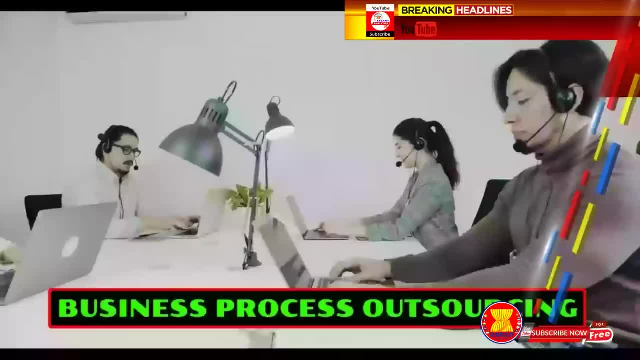 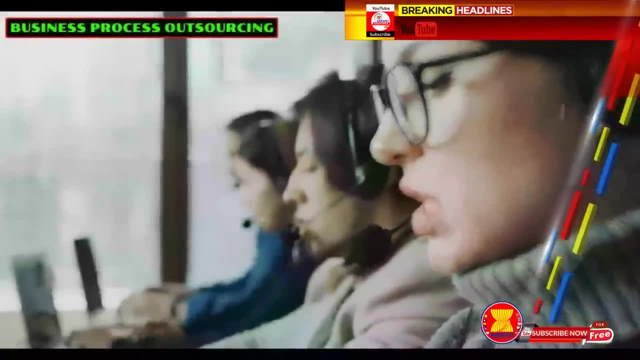 Within the service sector, business process outsourcing has played a significant role in sector growth. The Philippines was able to grow its BPO sector due to having professionals that spoke the languages necessary, partly due to the interest in US culture, of which the country is the. 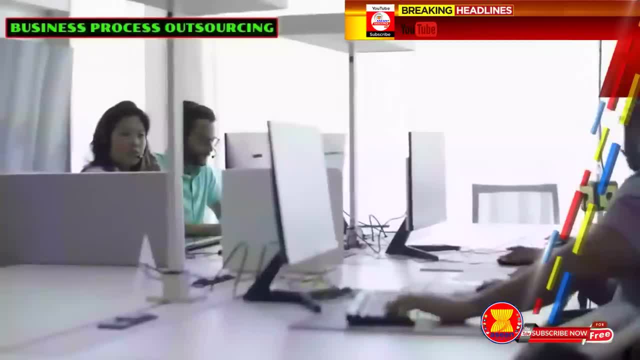 Philippines' largest BPO market And the customer service sector was able to grow its BPO sector due to having professionals that spoke the languages necessary, partly due to the interest in US culture, of which the country is the largest BPO market. 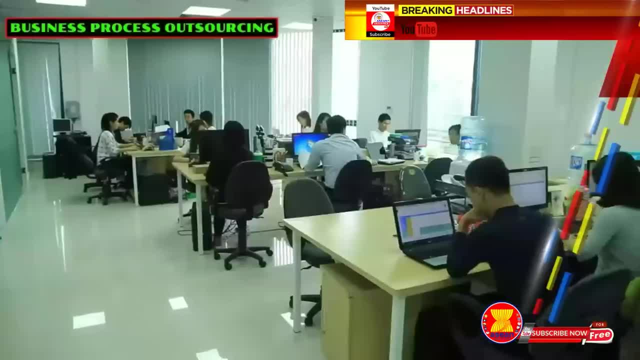 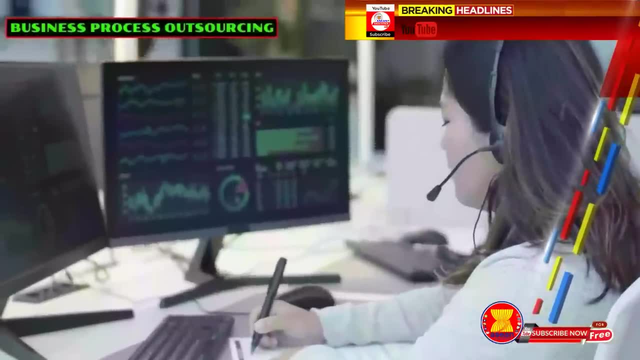 The BPO sector is a core service-focused aspect of the professionals in the industry. Supporting the growth and expansion of the ITBPM industry offers many opportunities for other industries. A buoyant outsourcing industry bodes positively well for the real estate sector as a result. 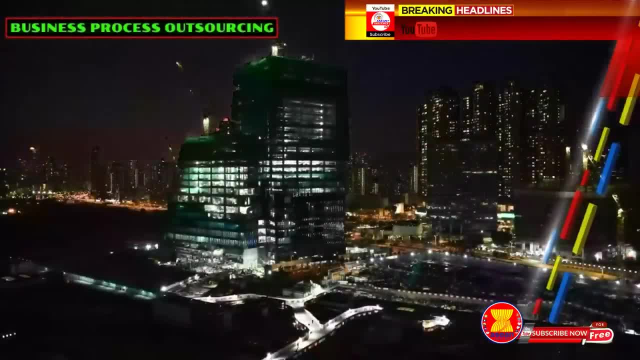 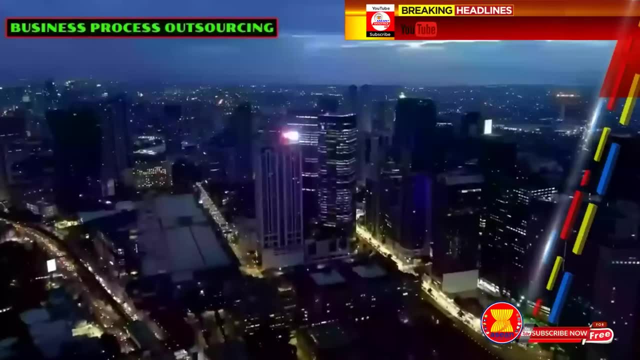 of increased demand for office space and residential condos. in addition to its benefits for the transportation, telecommunications, hospitality and retail sectors, The BPO industry, since its inception, has been a key part of the industry's growth. The BPO industry, since its inception, has been a key part of the industry's growth. 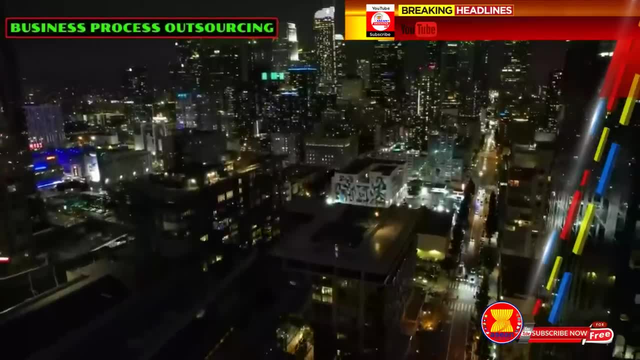 The BPO industry since its inception has been a key part of the industry's growth. The BPO industry since its inception has grown at rapid speed and has acquired significant traction in the global market share. This growth is attributable to the increasing demand of enterprises to reduce costs focus. 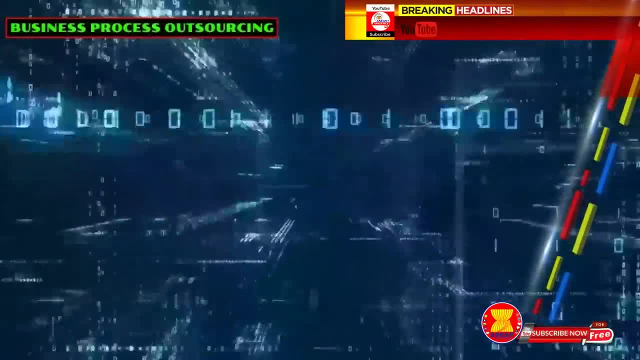 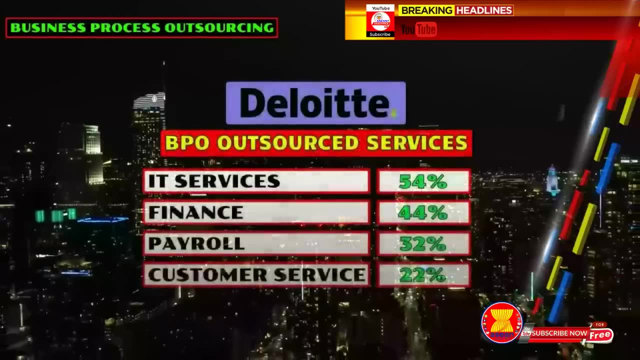 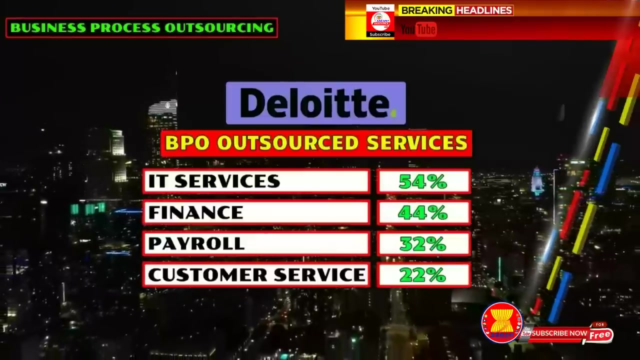 on their core business activities and handle problems such as a shortage of skilled personnel. Based on a 2021 report released by Deloitte, BPO-related enterprises include IT services at 54%, finance, payroll services and customer service or contact. 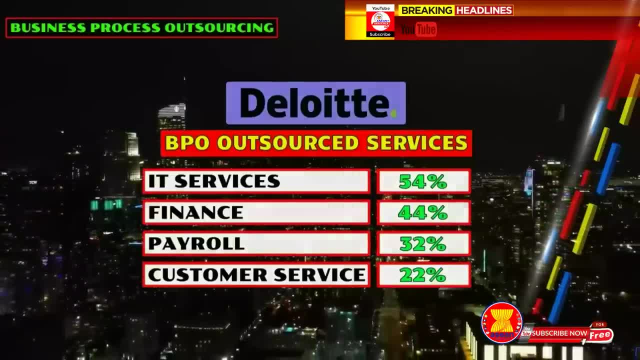 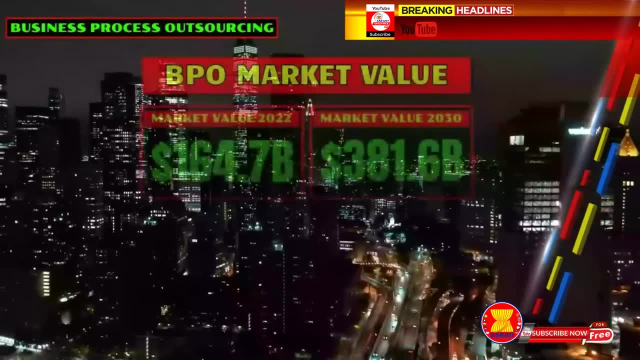 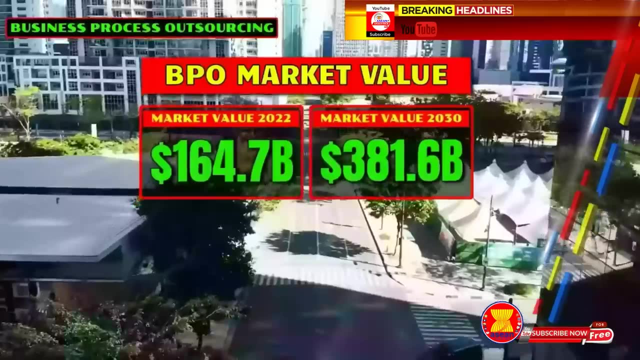 centers are the most often outsourced services. Despite the COVID-19 pandemic and recent economic headwinds, the global BPO industry has grown spontaneously, with an estimated value of $164.7 billion in 2022 and is expected to reach $381.6. billion by 2030.. According to IBPAP, the BPO industry currently employs 1,600,000 full-time employees and an expected $35 billion worth of revenue in 2023.. This is attributable to the pent-up demand from global customers. the higher confidence. 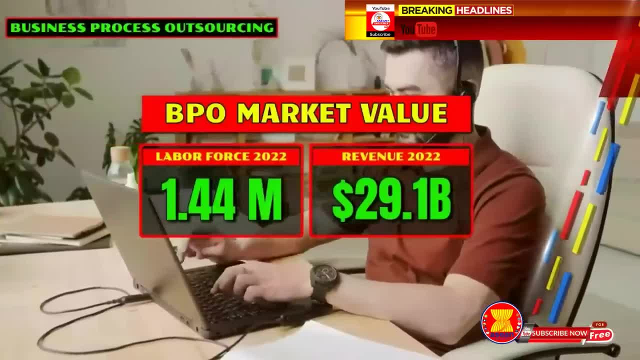 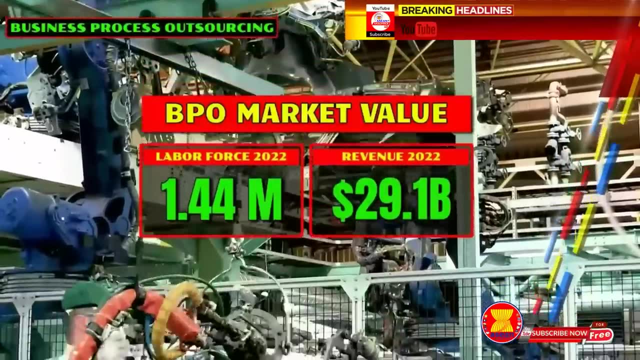 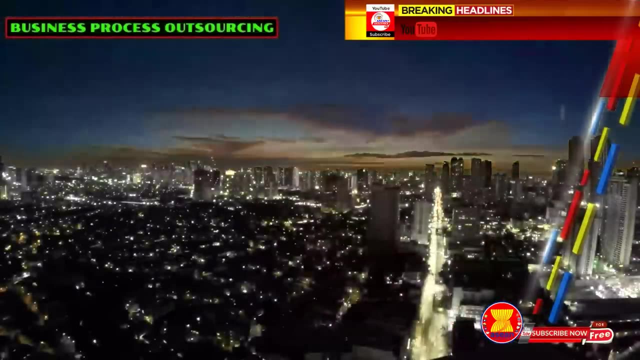 in a work-from-home setup by clients of contact centers and business process services, and growth in e-commerce, financial and healthcare technology. The BPO industry plays an important role in the Philippine economy's recovery from the pandemic. Although it was also adversely affected by the COVID-19 pandemic, the BPO industry has 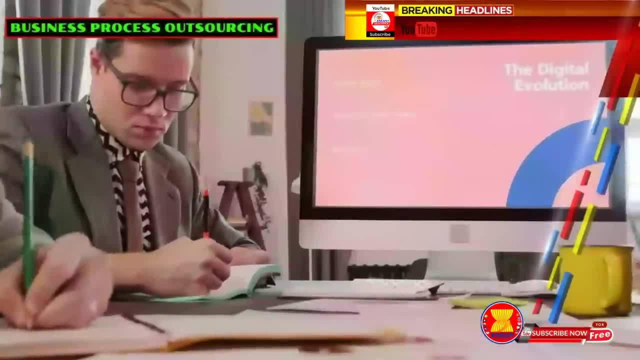 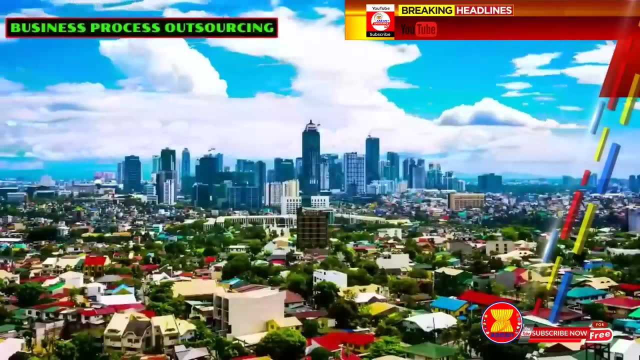 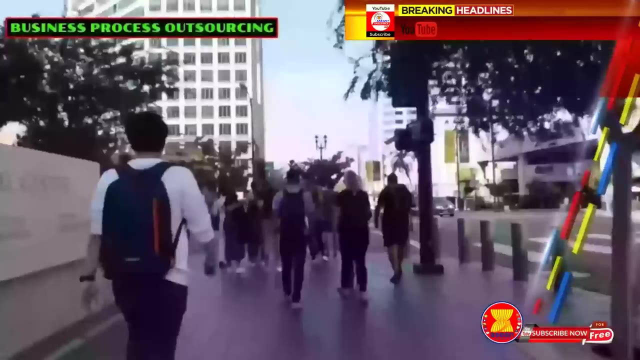 been a key part of the BPO industry since its inception. It adjusted relatively quickly and has invested in infrastructure that enabled it to keep its operations going. The industry's quick recovery is expected to spill over to 2030 and will continue to boost demand for ITBPM services, positively contributing to preserving jobs driving 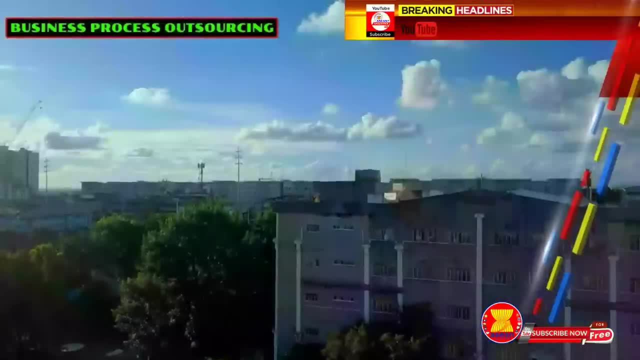 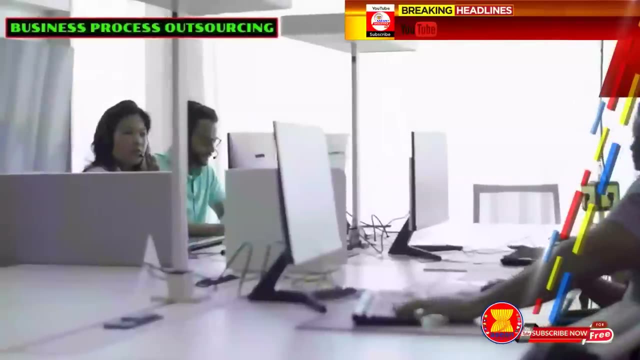 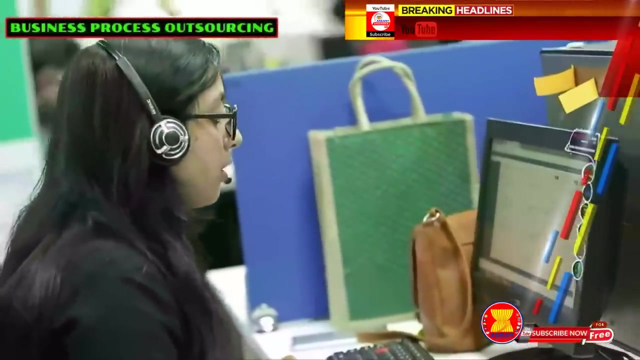 investment, stimulating countryside development and creating demand for real estate. Globally, India is the top player in outsourcing services. It is closely followed by the Philippines and the United States. India's BPO sector remains strong, offering 24-7 services and advances in technology. 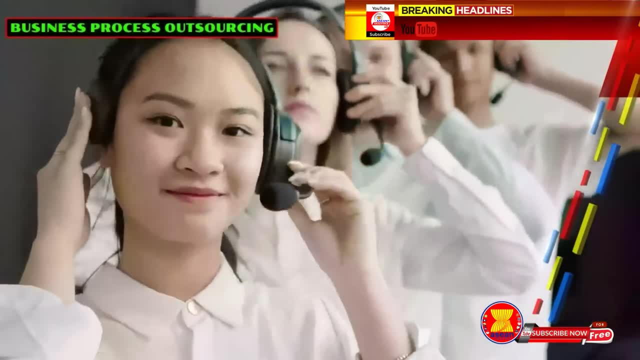 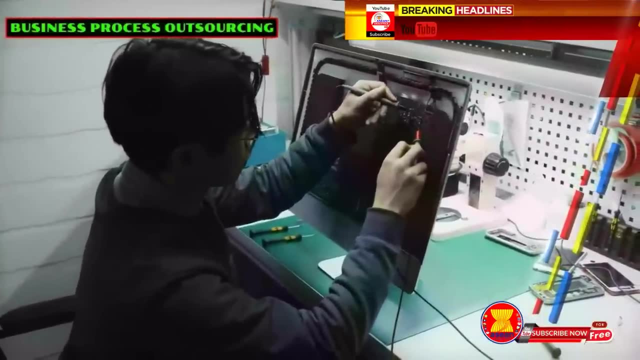 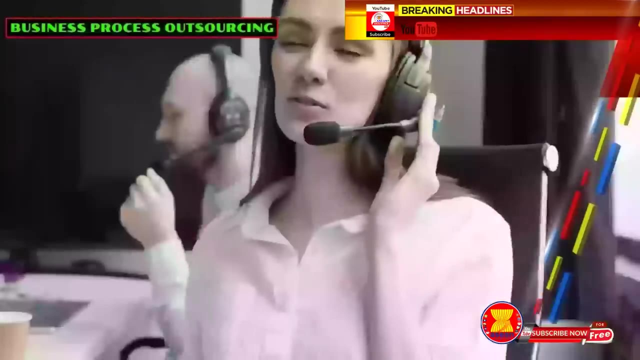 But in the voice or call center sub-sector, the Philippines have already surpassed India as a global leader since 2010.. While India is highly regarded for its IT expertise and impressive BPO-supporting infrastructure, Filipinos' soft skills, including customer support, English language proficiency and 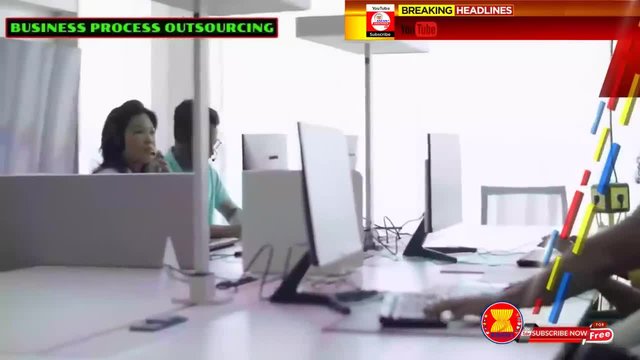 cultural affinity have been a key part of the BPO industry's growth. The BPO industry has a central affinity to the North American markets. are the Philippines' biggest draws which make the country a force to be reckoned with in the BPO sector? 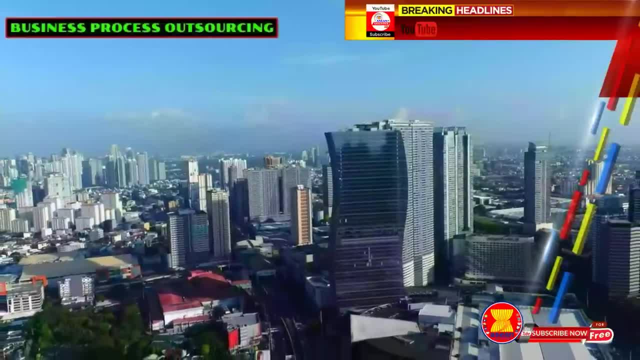 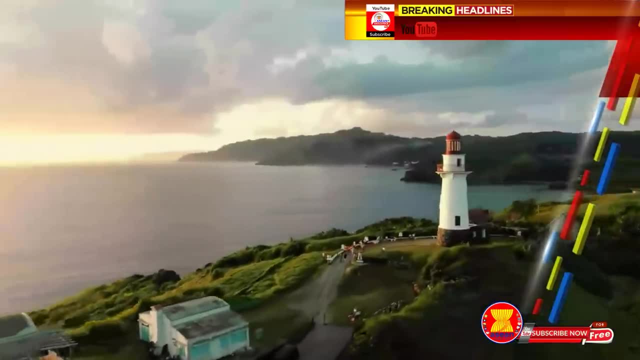 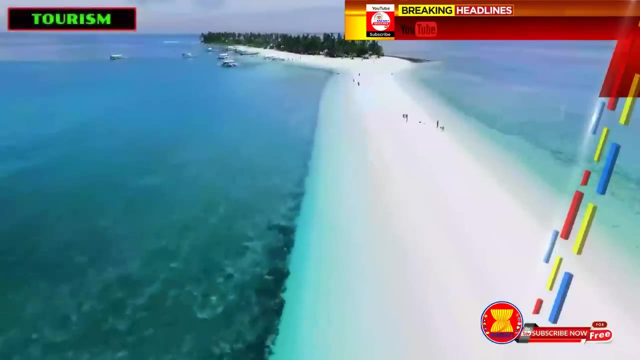 Today, the BPO industry in the Philippines holds an estimated 12-15% of the global BPO market. The second important segment within the service sector is tourism, which has a long history of moderate growth. Tourism in the Philippines has not been able to tap its resources optimally and has lagged. 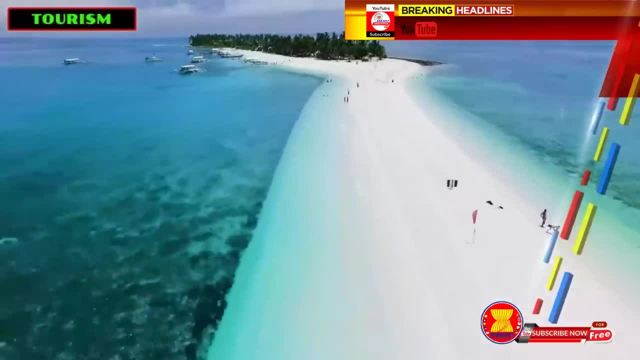 behind its regional cousins. Tourism in the Philippines has not been able to tap its resources optimally and has lagged behind its regional cousins. If tourism is not a major source of income for any country, it is a major source of wealth. The BPO industry has a major role to play in attracting international tourists, including 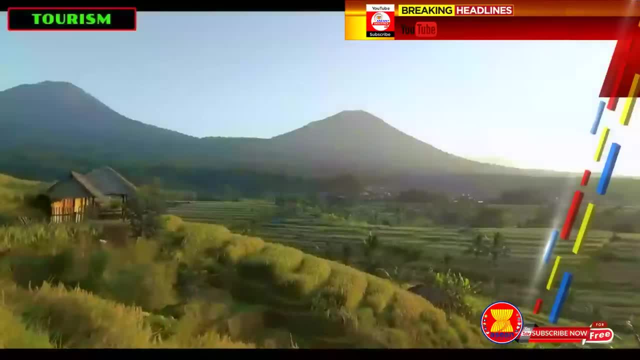 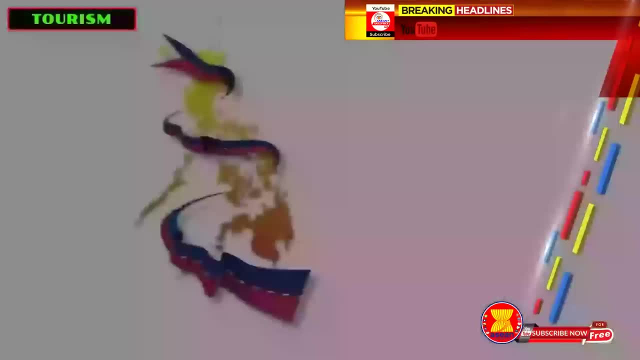 Singapore, Indonesia and Thailand. Inadequate infrastructure, poor rail and road connectivity and insufficient tourist services and facilities are among the chief reasons for this. However, with the $180 billion infrastructure project currently carried on, the Philippines' infrastructure will now be able to compete with regional peers. 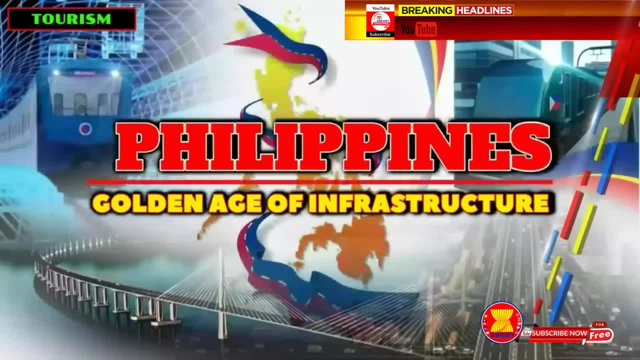 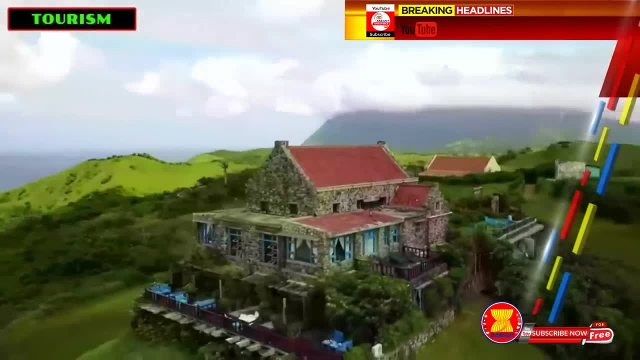 The country breached the 2,000,000-dollar US government capacity and provided a program for transportation in the Philippines, including a mobile system. marks in international arrivals for the first five months of 2023, surpassing last year's baseline. target, And these accounted for more than 100 billion pesos in estimated visitor receipts. International arrivals came from the United States, followed by South Korea, Australia, Canada, the United Kingdom, Japan, Singapore, India, Malaysia and China For 2023,. 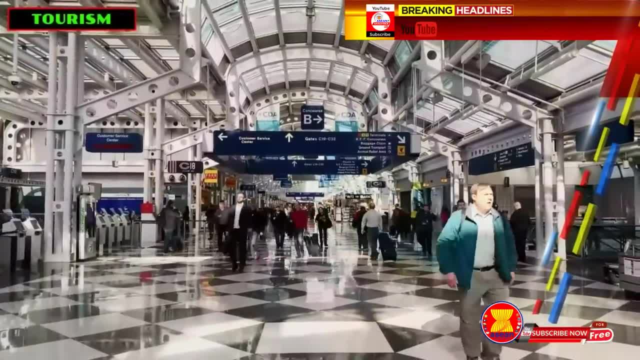 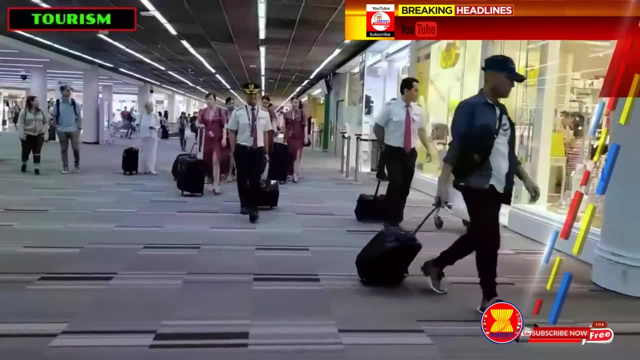 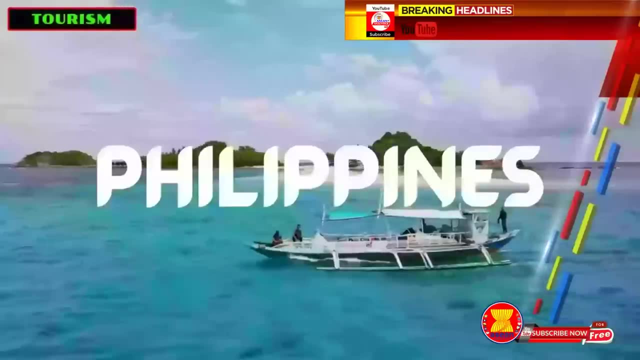 the Department of Tourism expects 4.8 million international arrivals and more than 120 million domestic trips as its baseline, But Philippine Tourism Secretary detailed, and remains hopeful, that the department will again surpass its targets, as it did in 2022.. The Philippines won several international recognitions, such as being the world's best country for a tourism. 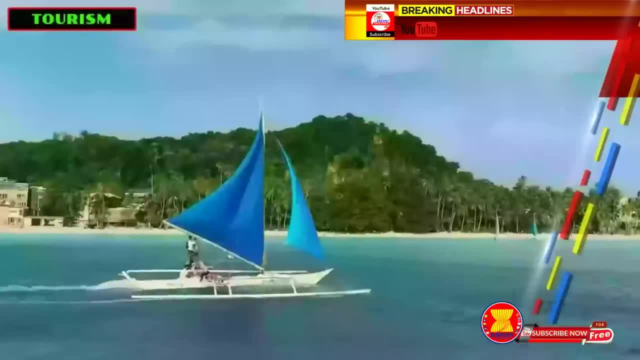 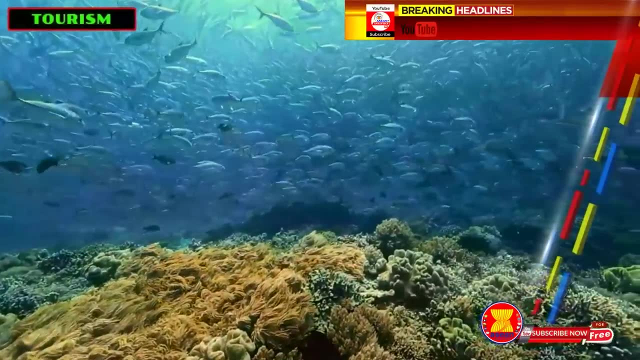 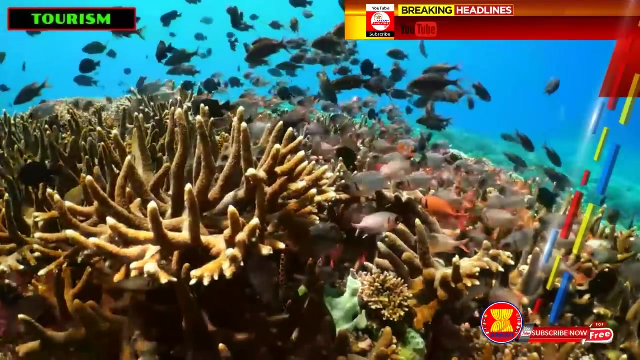 destination in the 2022 Wuzak Rota Global Travel Awards. World's leading dive destination 2022 by the World Travel Awards and other 13 awards in all categories available at Scuba Diving's 2023 Reader's Choice Awards by US-based Scuba Diving Magazine, including the top honors. 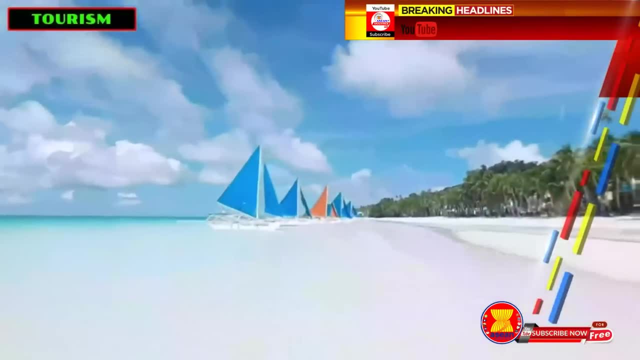 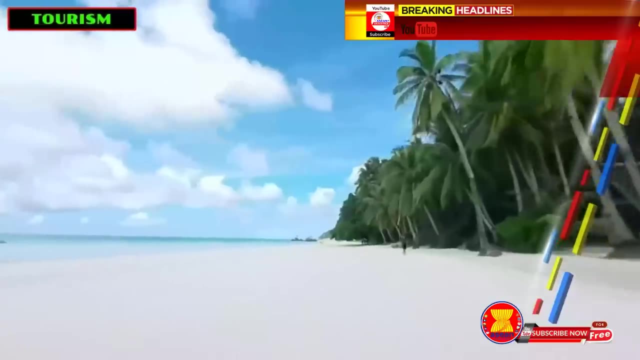 for shore diving Among the top tourist destination in the country is Boracay. Boracay Island's offering stage is its 4-kilometer-wide beach, prized for its incredibly inviting blue waters, fine white sand and perfect sunsets.